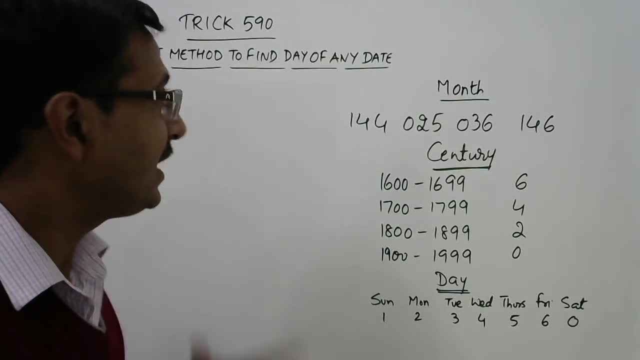 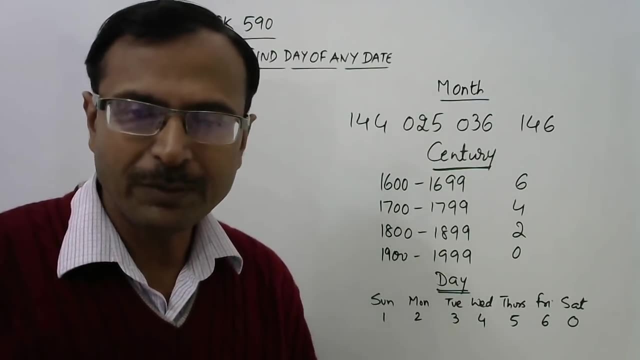 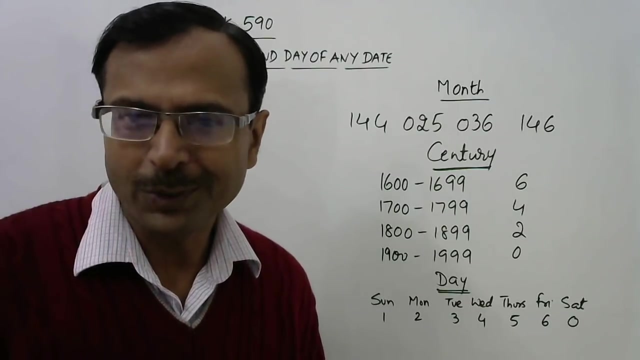 Hello friends, finding the day of any date a very, very common question in all kind of entrance exams. I posted one more video and you must have watched that. That video was little bit lengthy and so many of you pointed out that you know it took approximately 15 to 20 seconds. 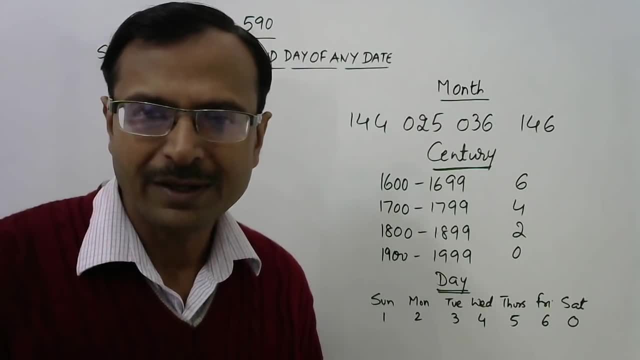 to get to the answer. So I thought of telling you a shortcut. This shortcut is devised to find the day of any date in less than 10 seconds. Well, I've tested it on some dates. You can do it and tell me whether this method is applicable on all dates or not. So for this we need to remember. 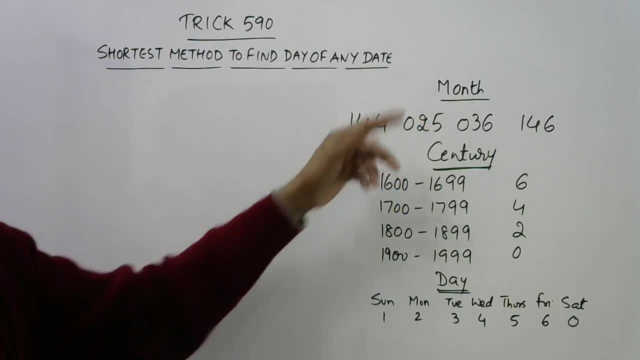 three concepts. See the month For the month, we have a number Like for January. we have 1, February 4, March 4, and so on December 6.. So I have distributed in triplets so that you can remember them easily, Actually. 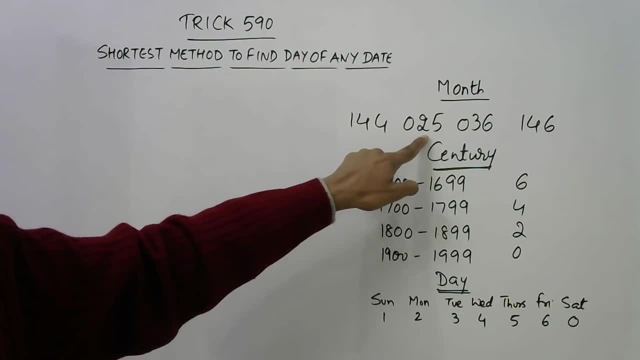 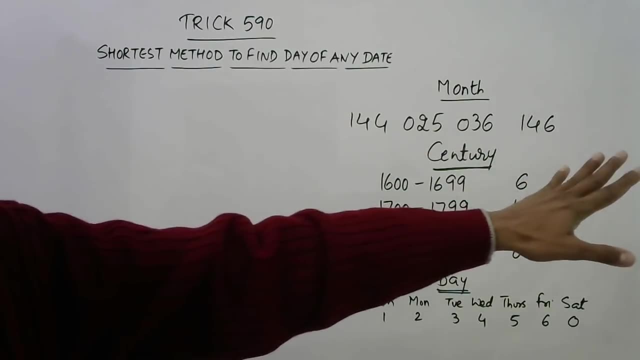 this is square of 12, 144.. Then 025 square of 5, 036 square of 6, and 144 plus 2 gives you 146.. So you can remember this: 144, 146, and in between you can have 5 square and 6 square. So these are. 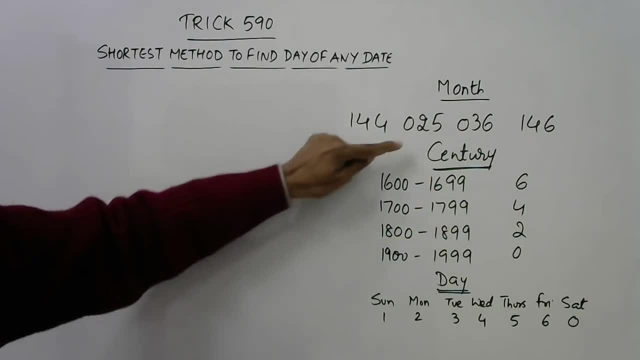 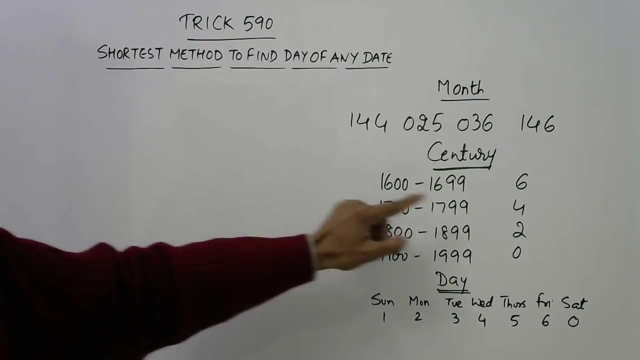 the 12 numbers for 12 months Now. for the centuries 1600, the century which starts with year 1600, that century, the number will be 6.. For the next century, starting with 1700, it will be 4.. Then, 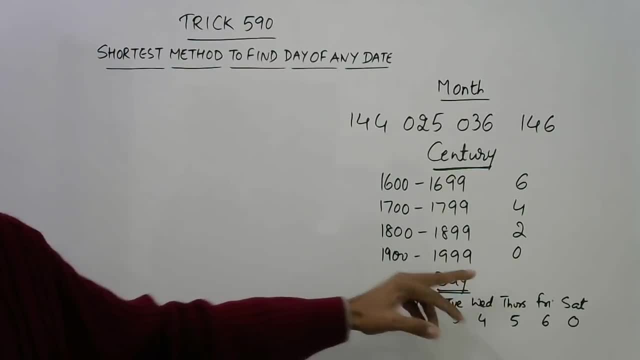 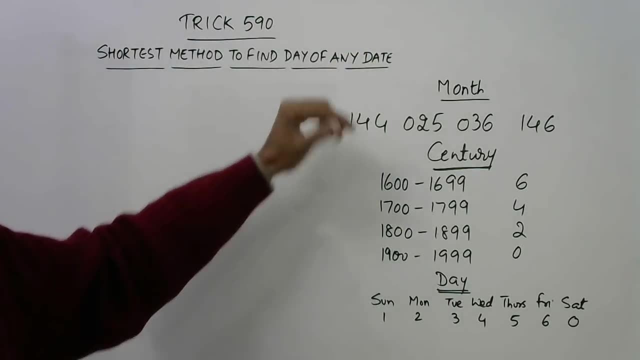 for 1800, it will be 2, and for 1900, it will be 0., And now you can repeat this 6402 for the successive centuries and preceding centuries also. So for 1500 to 1599, it will be 0. 1400 to. 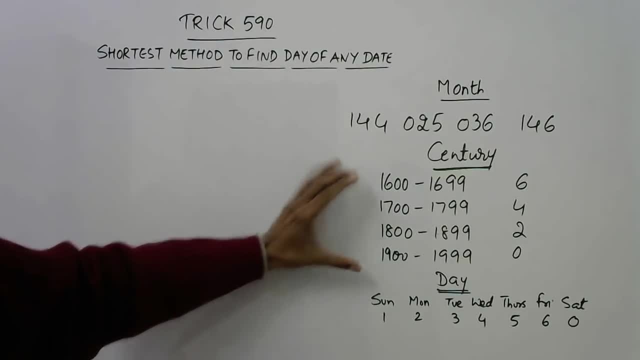 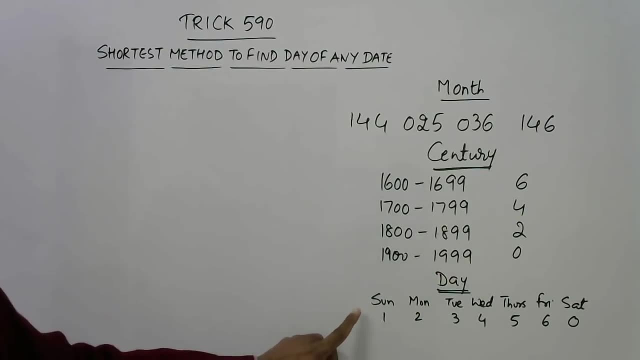 1499, it will be 2 and so on. So I have written 4.. You can extrapolate this for more years, more centuries before and after this. For days, we have the numbers 1 to 6, followed by 0. So it starts from Sunday 1, Monday 2,. 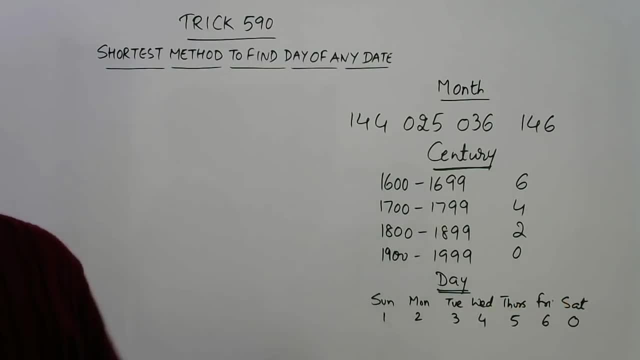 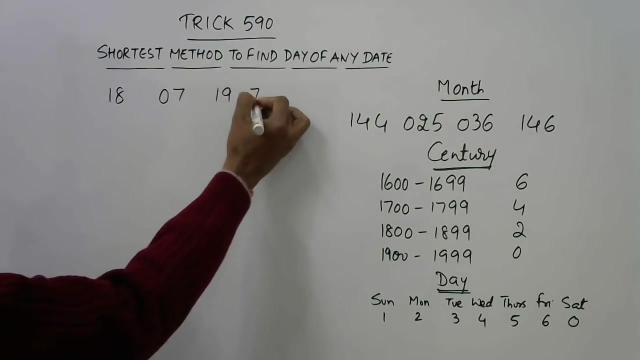 Tuesday 3 and goes up to Friday 6, then Saturday 0.. So these are the 3 things you need to remember and I will apply it on 2 dates and then you can solve it using some other dates and tell me whether it is right or not. So I am taking my birthday, 1807, 1973. So I have written. 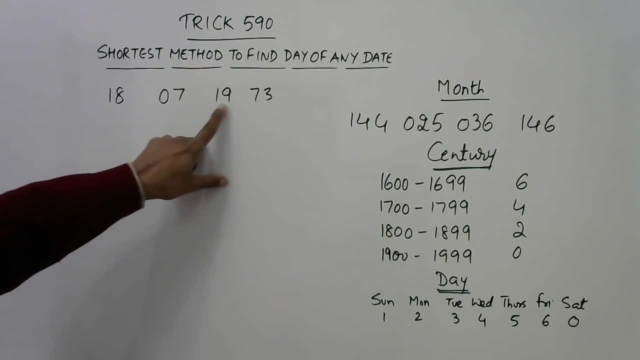 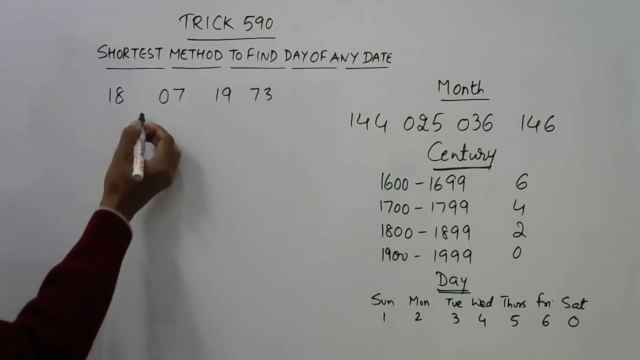 4 numbers here. This is the date, this is the month, this is the century and this is the year. This is the year of the century, So 18071973.. Now this for this. the first number is 18,. 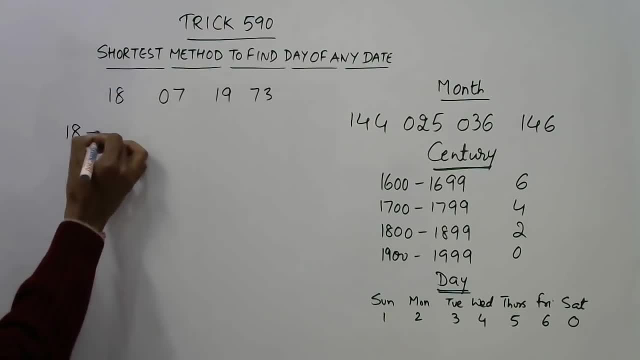 that is the date. So 18 will come as it is. Plus, I will have one more number, followed by one more number, followed by the fourth number here: 73.. So the first number is same, fourth number is same: These 2 numbers corresponding to these 2 numbers, we will have 2 numbers. 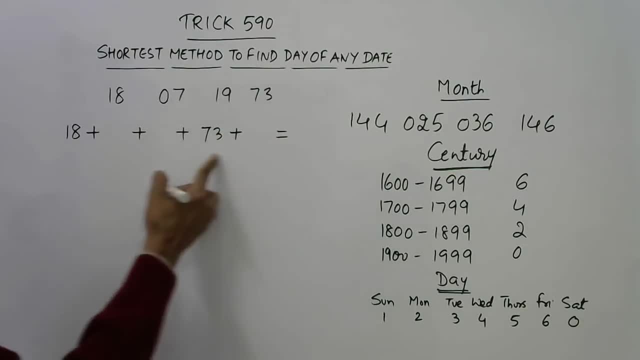 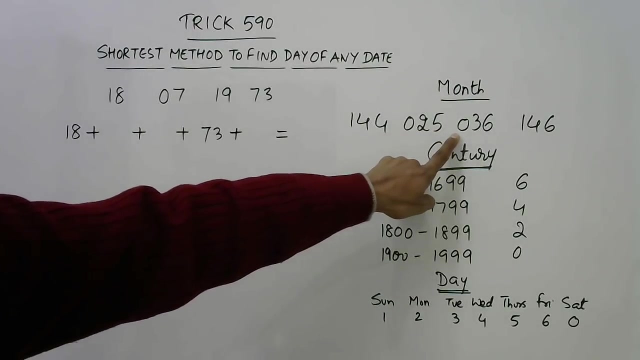 here. and finally one more number. then the sum of these will be written on the right hand side. Now see 18. we have already written here. Now this is the month 7th month. Then 7th month corresponding to month, we have 1,, 2,, 3,, 4,, 5, 6, 7.. 7th number is 0., So you. 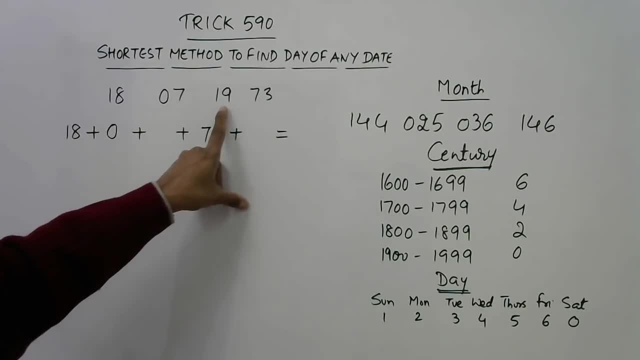 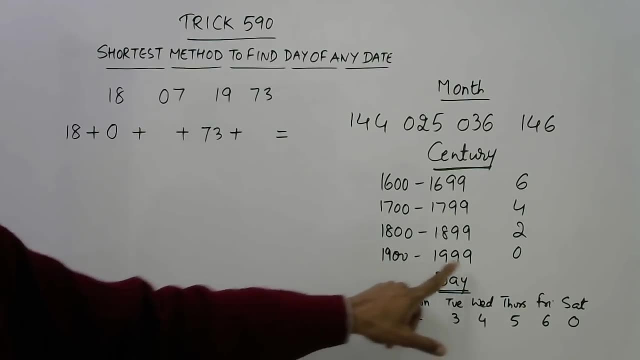 write 0 here, Then, corresponding to the century, that is 19.. It starts with 1900 to 1999.. So year lies between this. So the corresponding number is 0.. Now I look at this number: 73.. 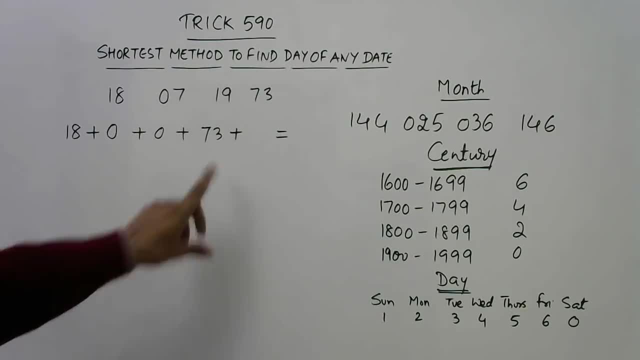 Try and divide this number, 73, by 4.. So if you divide this by 4. So I will write it here for you- 73 divided by 4 gives you a quotient of 18.. 18 for the 72.. So the quotient. 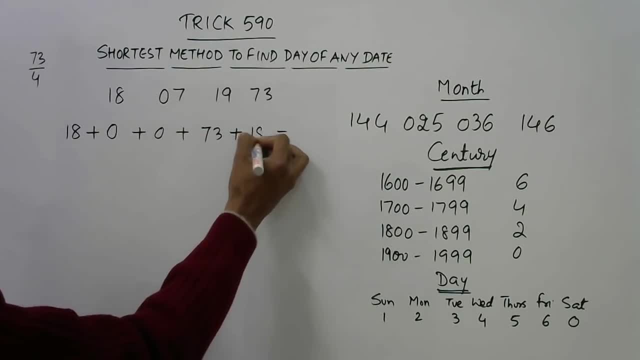 is to be written here. So 18 for the 72.. So, on dividing this number by 4, you have 18 as the quotient, And now add all the numbers 73 plus 18 is 91,, 114 plus 7,, 9,, 6, 7,, 8,, 7, 7.. So this: 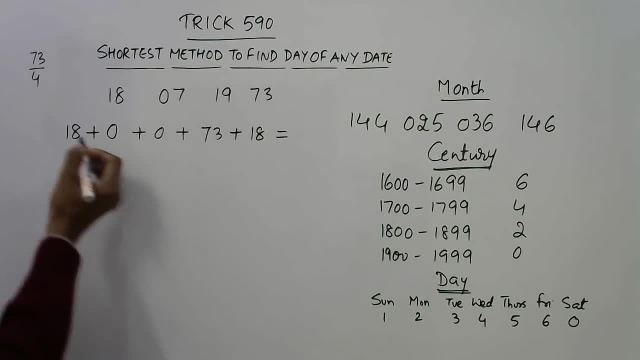 is the quotient. So we have gone through all of these. So this is the quotient of this number. So let's, 101,, 101,, 109 is the result. And finally, whatever number you obtain on adding these 5 numbers, just divide it by 7.. So, remember, this number has to be divided by 4 and quotient.